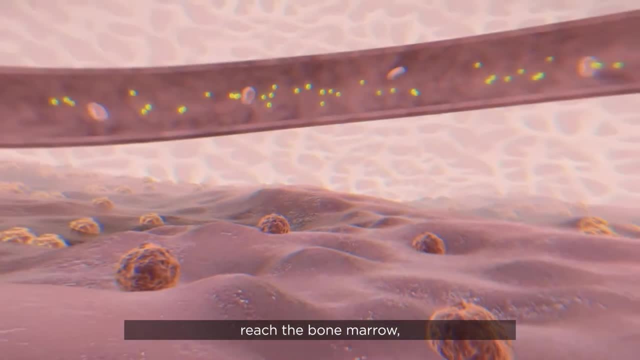 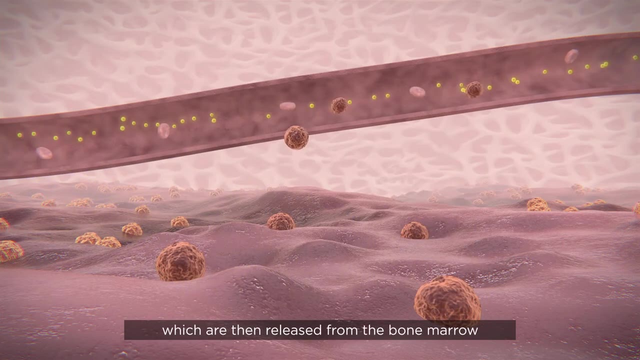 the compounds released by the injured tissue reach the bone marrow. these messengers tell the stem cells in the bone marrow to divide and create new stem cells, which are then released from the bone marrow into the bloodstream. Slowly, the number of stem cells increases. 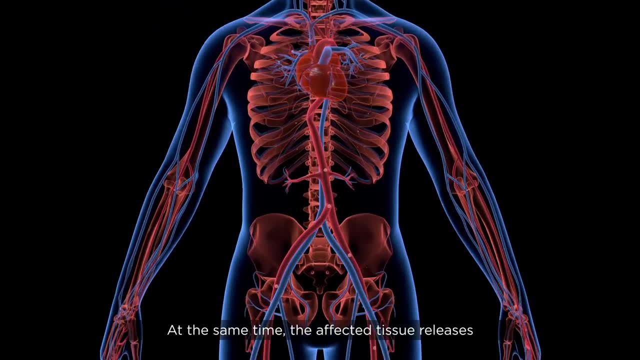 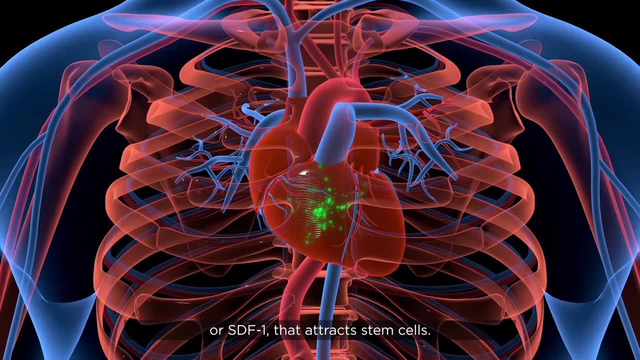 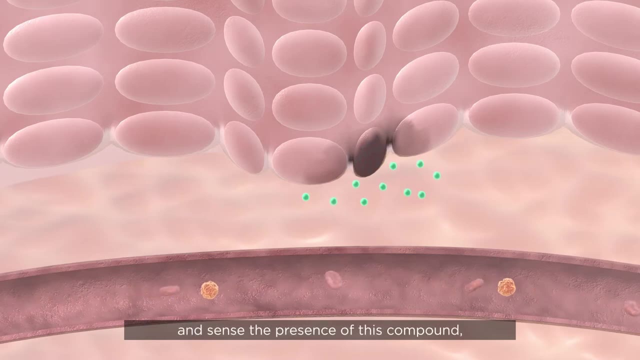 in the blood circulation. At the same time, the affected tissue releases another compound called stromal-derived factor 1, or SDF1, that attracts stem cells, As stem cells circulate in the fine blood vessels of the affected tissue and sense the presence of. 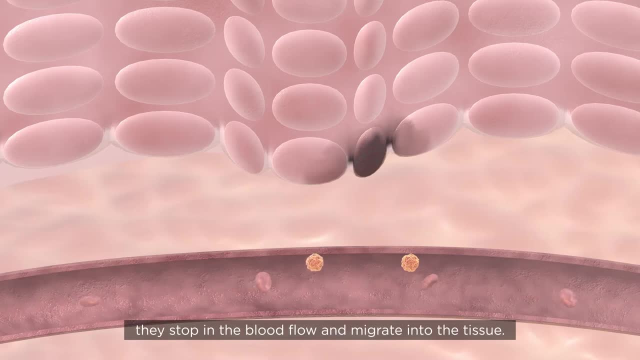 this compound, they stop in the blood flow and migrate into the tissue Inside. the tissue stem cells slowly migrate to the very site of injury where SDF1 is being secreted. When they reach the site of the injury and come into contact with the damaged, tissue, stem cells begin to multiply and 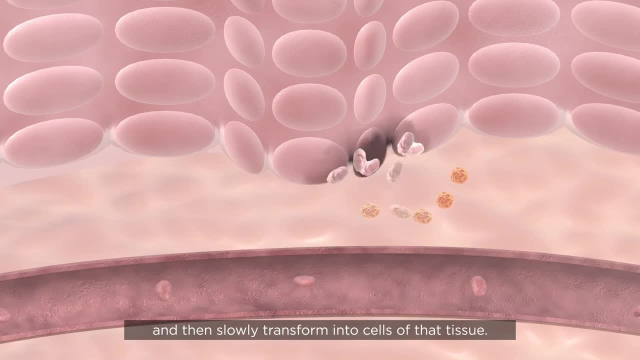 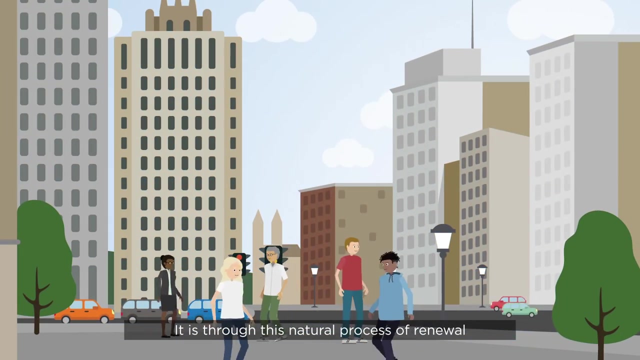 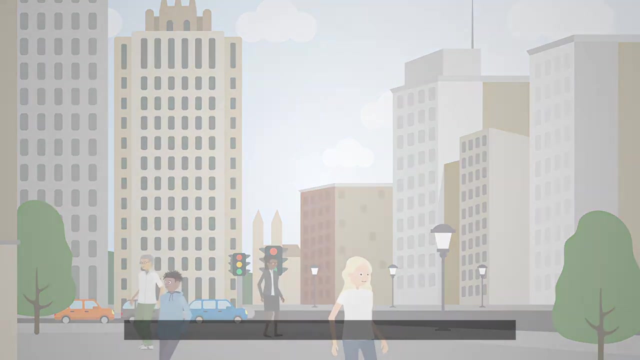